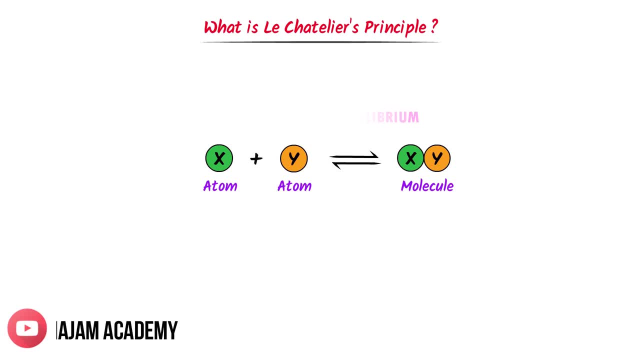 the chemical equilibrium. Let consider that I add one another atom of X and one another atom of Y, So I have changed the concentration of reactants. Now this system will respond to this change of concentration of reactants. Let me repeat it: This system will respond to this change of concentration of reactants. 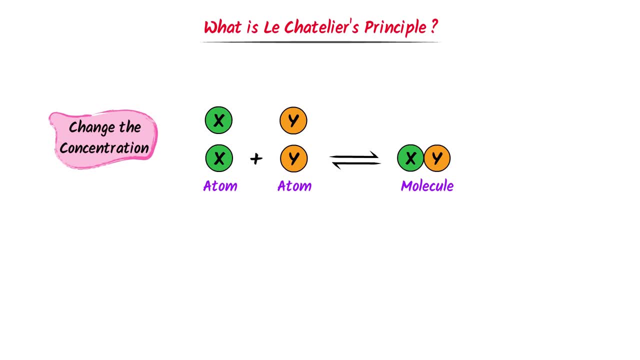 Here the change is simple. I mean, the concentration of reactants is large and the concentration of product is small. So what will be the response of this system? It is very simple. The rate of forward reaction will become high to make more products. Now, the rate of forward. 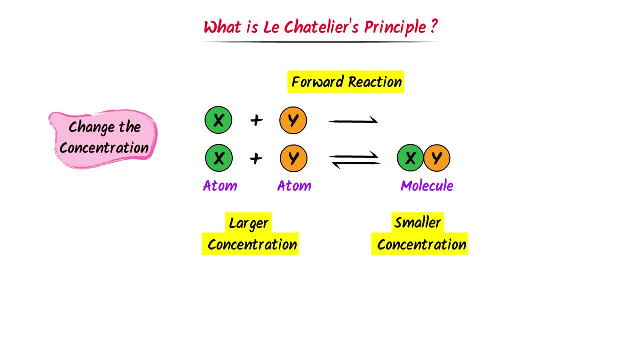 reaction is higher than the rate of backward reaction, Or we say that equilibrium is shifted in forward direction. Lastly, when two molecules are completely formed, the system will restore its chemical equilibrium. I mean, the rate of forward reaction becomes equal to the rate of backward reaction because four atoms react. 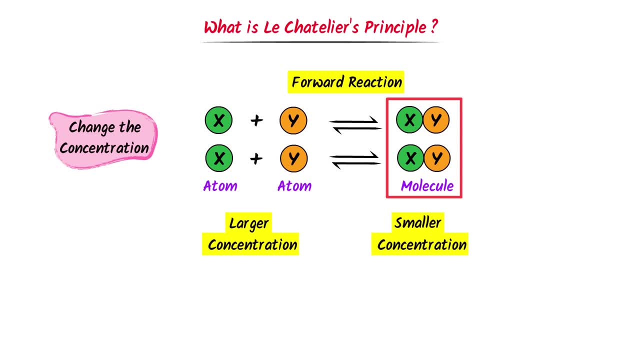 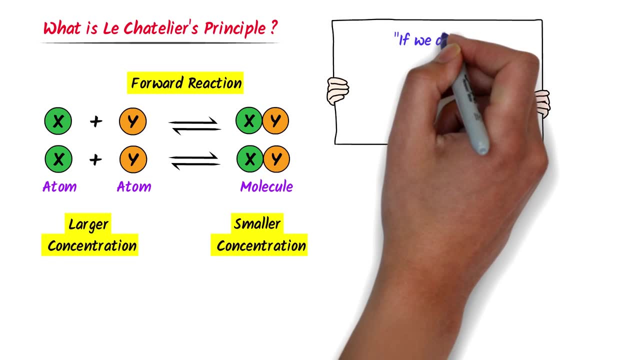 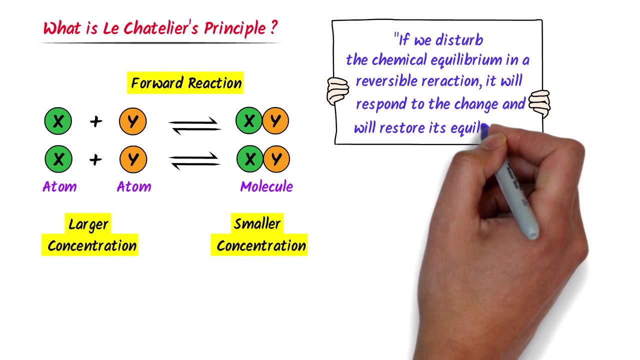 together to form two molecules, and two molecules break down to form four atoms. Now listen carefully. Overall, we learn that If we disturb the chemical equilibrium of a reversible reaction, it will respond to the change and will restore its chemical equilibrium. Let me repeat it. 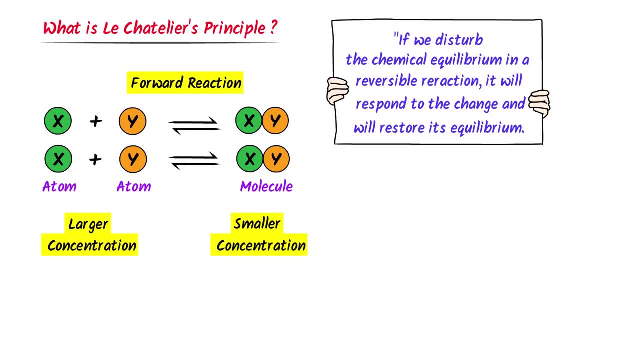 If we disturb the chemical equilibrium of a reversible reaction, it will respond to the change and will restore its chemical equilibrium. This is what the Lee-Chet Lear's principle state. So note it down, this super easy definition of Lee-Chet Lear's principle, which is often 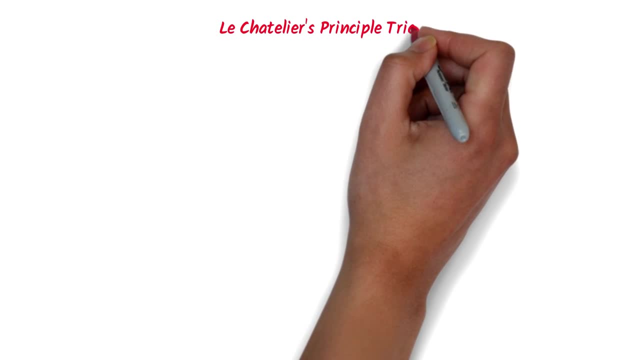 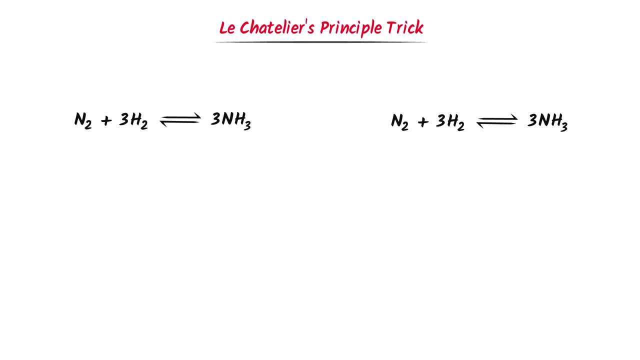 made very difficult. Now let me teach you my personal trick of Lee-Chet Lear's principle, For example. consider these reversible reactions Now. what will happen if we increase the concentration of hydrogen gas, in this case, and decrease the concentration of nitrogen gas, in this case? 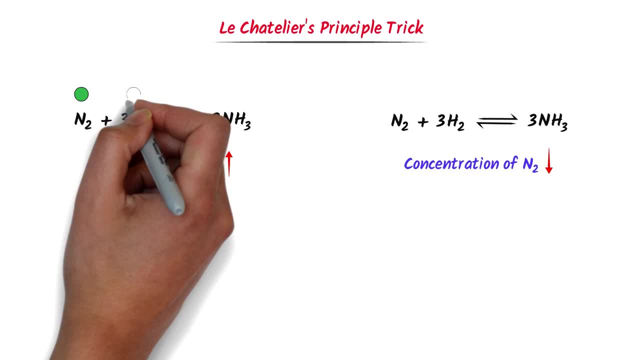 Well, I use my personal trick. Let X atom and Y atom react together to form XY molecule, and XY molecule breaks down to form XY atoms. Now listen carefully. When we increase the concentration of hydrogen gas, it means that we are adding more hydrogen. 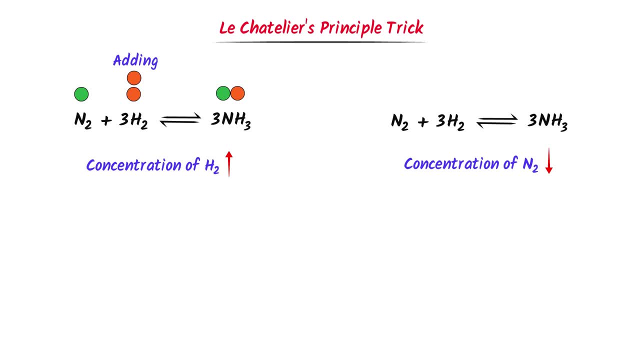 gas Here. if I ask you what is changed, Your answer is simple: There are more reactants and less product. Secondly, if I ask you what is the response of this system, Your answer is again simple: The equilibrium will proceed. 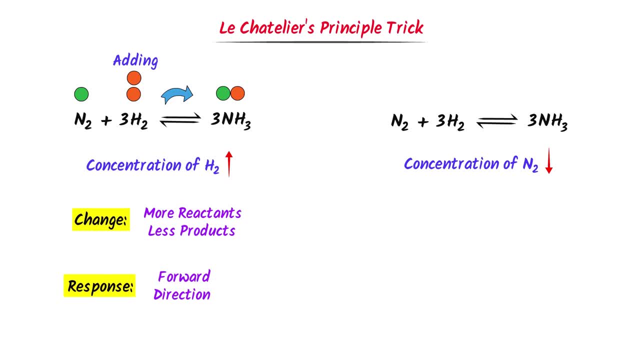 In forward direction to form more products and neutralize the effect of concentration. Let me repeat it: The equilibrium will proceed in forward direction to form more products and neutralize the effect of concentration. Therefore, remember that if we increase the concentration of the hydrogen gas, equilibrium 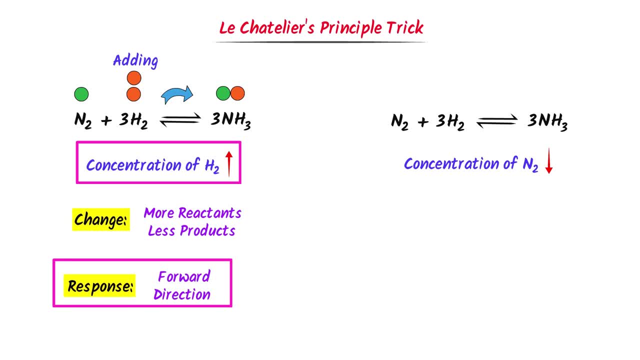 will shift in forward direction to neutralize the effect and restore chemical equilibrium. Secondly, I again write X and Y atoms. they react together to form XY molecule. Now listen carefully. When we decrease the concentration of nitrogen gas, it means that we are reducing or removing. 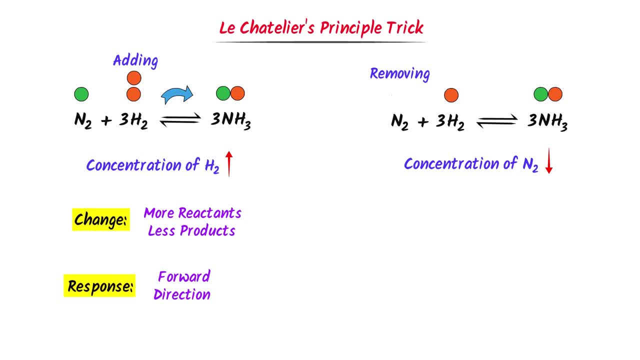 nitrogen gas Here. if I ask you what is changing and what is the response of the system, Your answer is simple: There are more products and less reactants. Secondly, the equilibrium will proceed In backward direction to form more products and neutralize the effect of concentration. 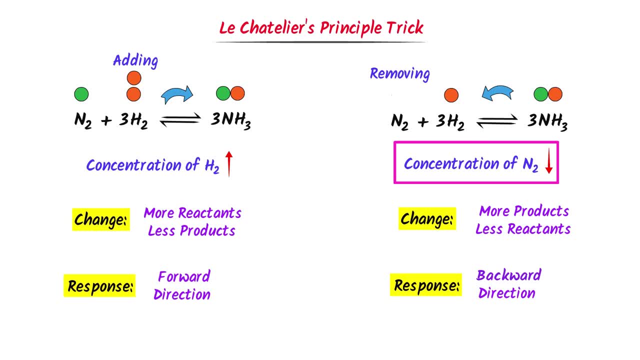 Therefore, if we decrease the concentration of nitrogen gas, equilibrium will shift in backward direction to neutralize the effect and restore chemical equilibrium. Thus, using this trick, we can easily calculate the equilibrium shift if concentration is changed. Now let me teach you the effect of changing pressure. 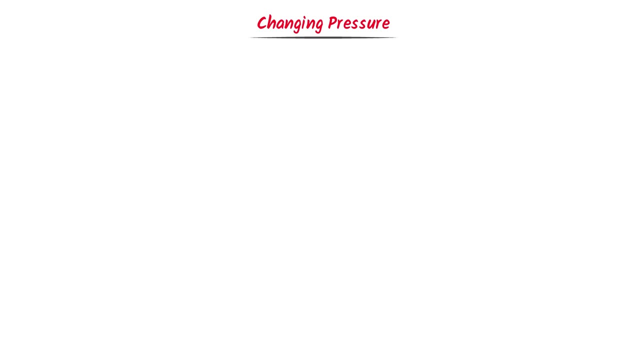 Here. remember that changing pressure only effects reversible reactions if reactants and products are in gaseous state. Now consider these reactions. What will happen if we increase the pressure in this case and decrease the pressure in this case? Well, on the left side there is 1 mole of PCl5, while on the right side there is 1 mole. 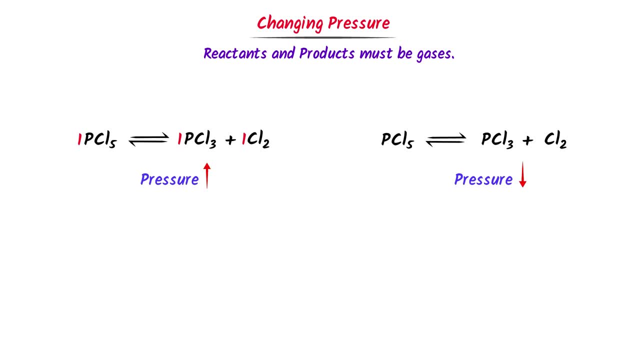 of PCl3.. So I write 1 mole of reactants and 2 moles of products. Now here the trick is that we only consider larger number. We can see that the larger number is 2 mole. Now listen carefully. 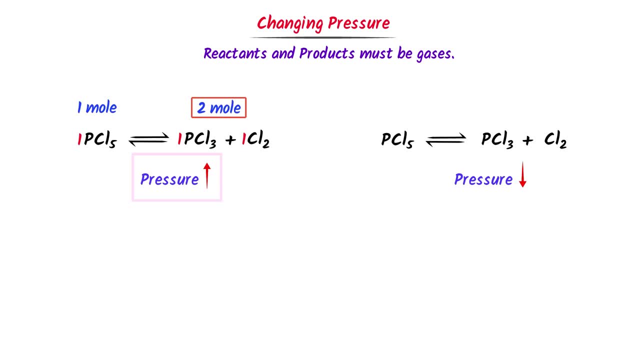 When we increase the pressure, it means that we are increasing the number of 2 moles further and putting more pressure. Let me repeat it: When we increase the pressure, it means that we are increasing the number of 2 moles further and putting more pressure. 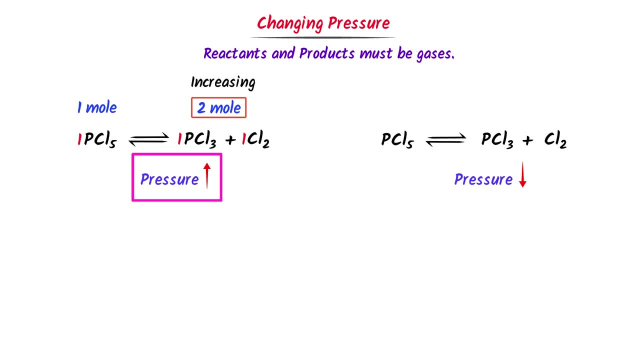 Let me repeat it: When we increase the pressure, it means that we are increasing the number of 2 moles further and putting more pressure. So here the change is more pressure on products and less pressure on reactants. Can you guess the response of this system? 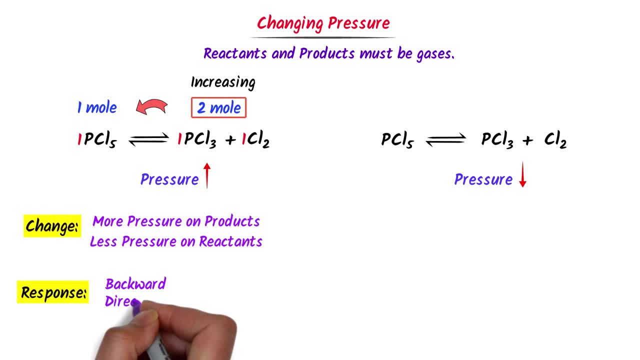 Well, it is simple. The equilibrium will proceed in backward direction to counter the effect of pressure and restore chemical equilibrium. In this case, we already know that there is 1 mole of reactants and there are 2 moles of products. We know that we only consider the larger number. 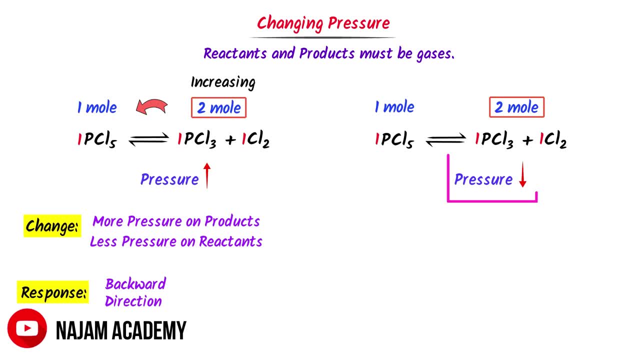 Here the larger number is 2.. Now, when we decrease the pressure, it means that we are decreasing the number of 2 moles further and putting less pressure on reactants. Let me repeat it: When we decrease the pressure, it means that we are increasing the number of 2 moles further. 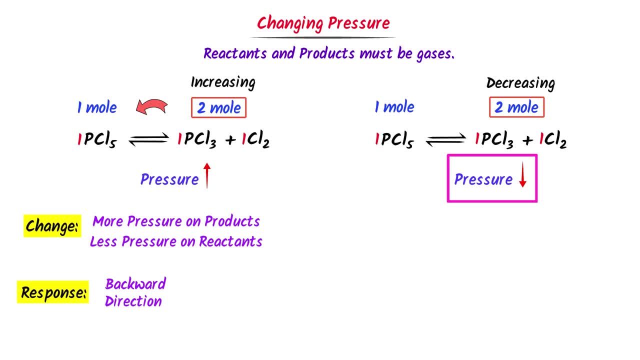 and putting less pressure on reactants. It means that we are decreasing the number of 2 moles further and putting less pressure on reactants. So here the change is less pressure on products and more pressure on reactants. Thus the response will be: the equilibrium will proceed in forward direction to counter. 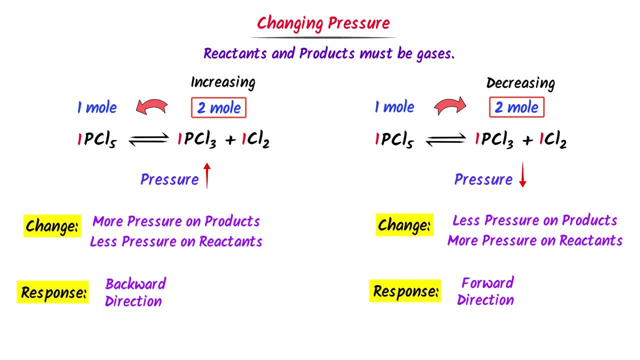 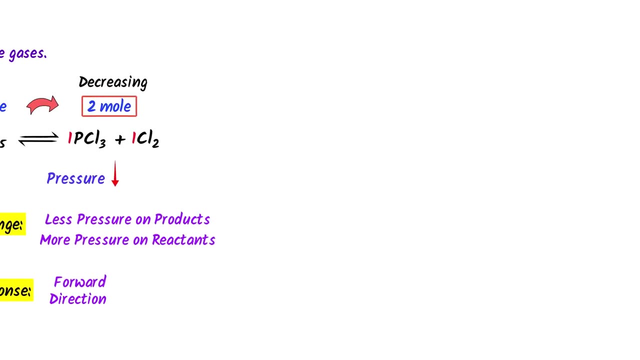 the effect of pressure. Therefore, remember that decreasing pressure means that equilibrium will shift in forward direction. So using this simple trick, we can easily calculate the effect of change of pressure on chemical equilibrium. Here let me teach you one bonus question. Consider this reversible reaction. 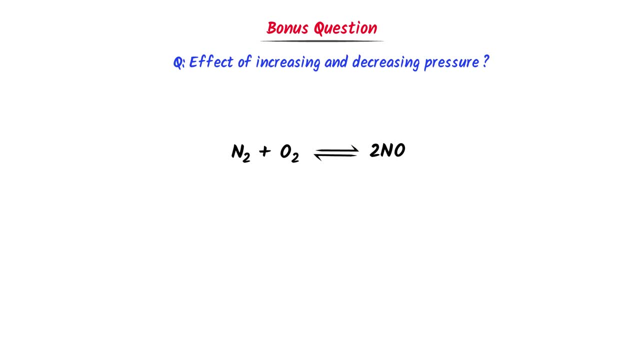 What will be the effect of increasing or decreasing pressure? Well, the answer is simple: Increasing or decreasing pressure has no effect on this chemical reaction, because the number of moles of reactants is 2.. And the number of moles of reactants is 2.. 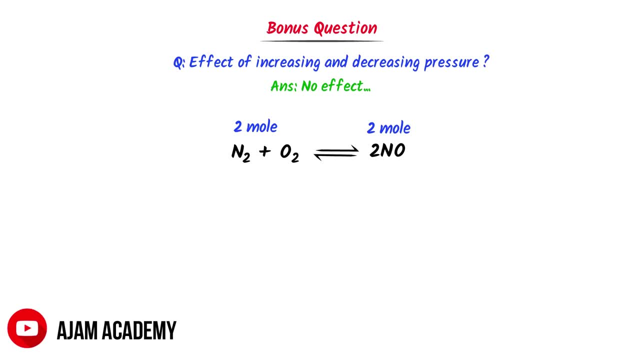 So the reaction will be the same. The number of moles of products is also 2. So note it down that if the number of moles of reactants is equal to the number of moles of products, changing pressure doesn't affect the chemical equilibrium. 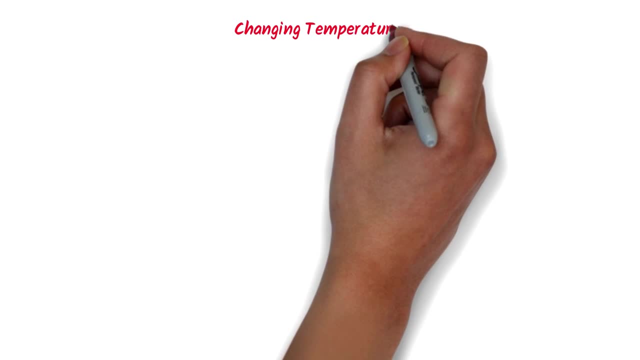 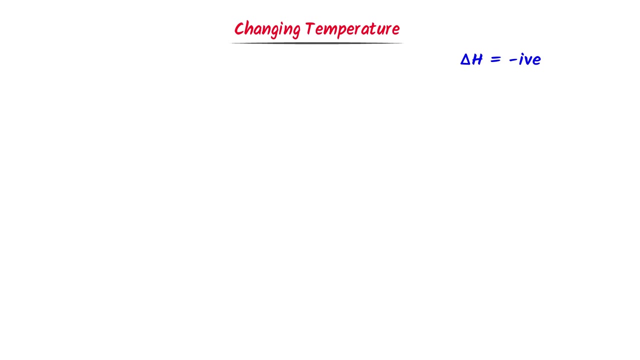 Finally, let me teach you the effect of changing temperature on chemical equilibrium. Remember that if heat of enthalpy del H is negative, it is an exothermic reaction in which heat is given off to the surrounding, While if heat of enthalpy is negative, it is an exothermic reaction in which heat is. 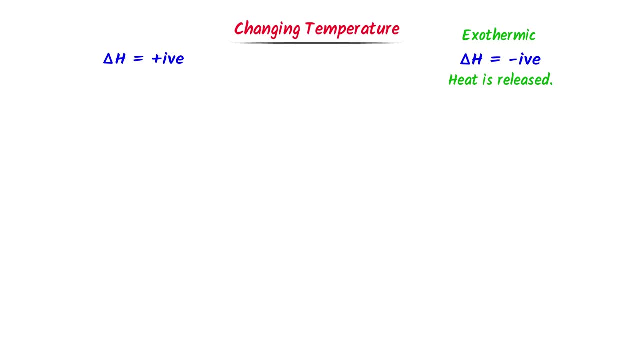 given off to the surrounding. While if heat of enthalpy del H is positive, it is an endothermic reaction in which heat is absorbed from the surrounding. Now consider these reversible reactions. What will happen if we decrease temperature in this case and increase temperature in this? 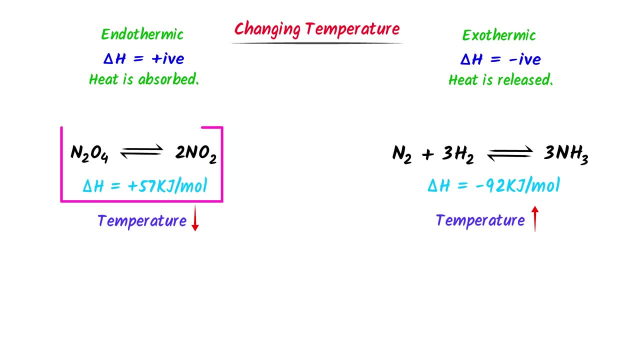 case. Well, we know that this is endothermic reaction. In case of endothermic reaction, I always write here cold And I write here hot. Here the trick is, we only consider the hot side and we do not look at the cold side. 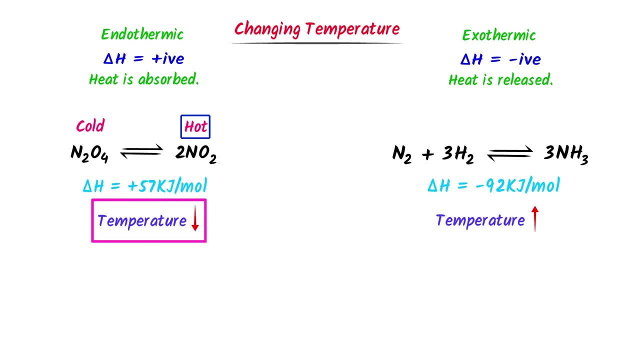 Now listen carefully. If we decrease the temperature, it means that we are cooling the hot side or removing heat from the hot side. Let me repeat it: If we decrease the temperature, it means that we are cooling the hot side or removing heat from the hot side. 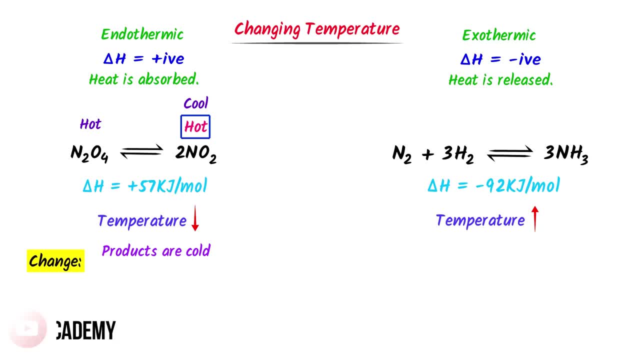 So the change in temperature is negative. The change is: product becomes cold and reactants become hot. Now the response is: equilibrium will proceed in forward direction in order to produce more reactants to counter the effect of temperature. Secondly, in this case we know that the enthalpy of heat is negative, so it is an exothermic.